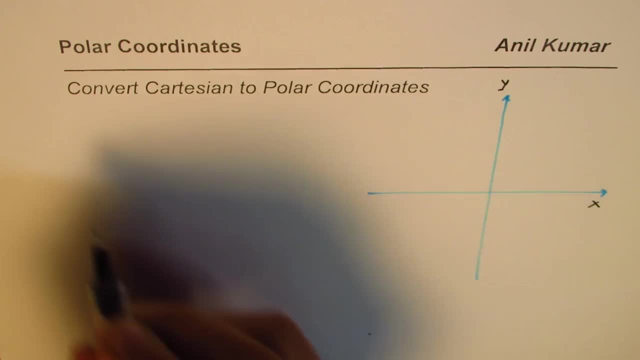 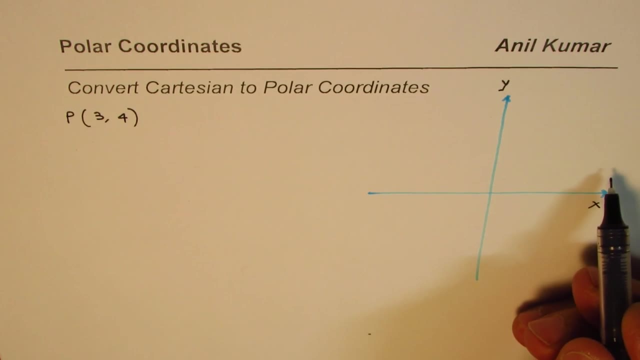 Now, as an example, let me take a point. Let's say the point P given to us is 3, 4.. So if that is the point in a cartesian plane, we'll see how to convert this on the polar coordinate system. 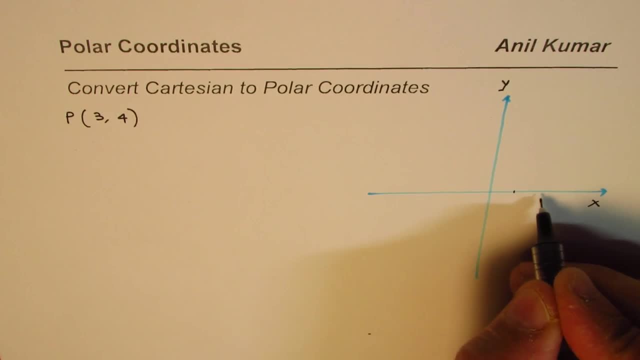 right. So point P, which is 3, 4, really means you move 1,, 2,, 3 units along the x. Y is vertical, right, So move 4 units along the y. That means 1,, 2,, 3, and 4.. You get to the point and this point. 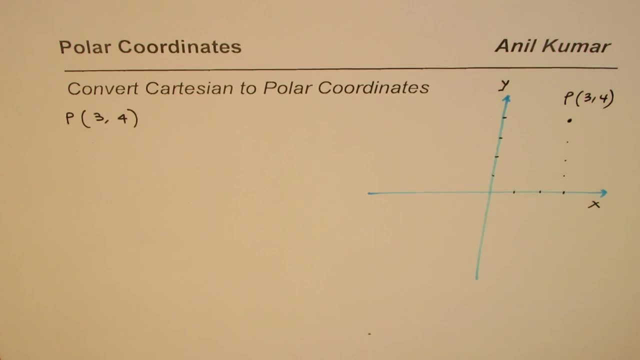 P is 3,, 4, right. So that is how you get a point on the polar coordinate system, I mean on the cartesian point. right Now, if I have to convert it to polar coordinate system, what do I do? So I make another scale. Let me think that we have put the scale on this. 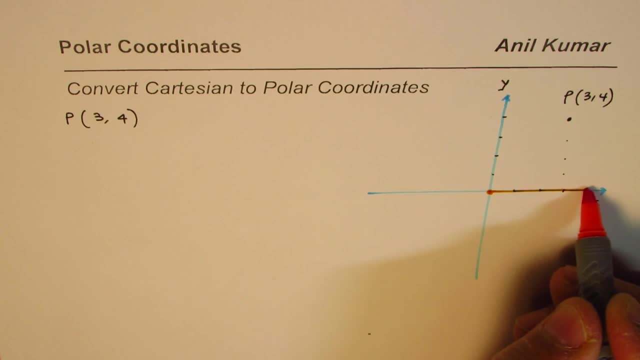 So it will have a pole here and the polar axis, right. So this becomes the polar axis, And to represent the point, we'll just connect this point with the pole like this And we say: well, that is the polar coordinate, right. 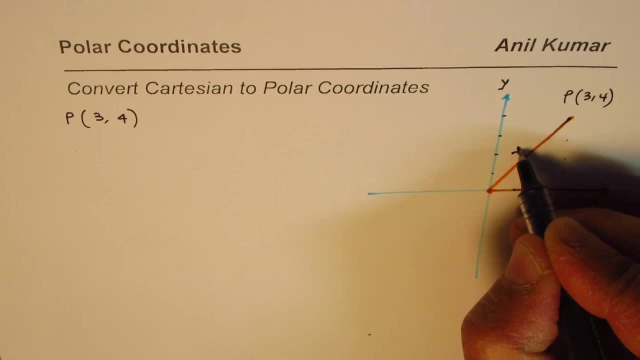 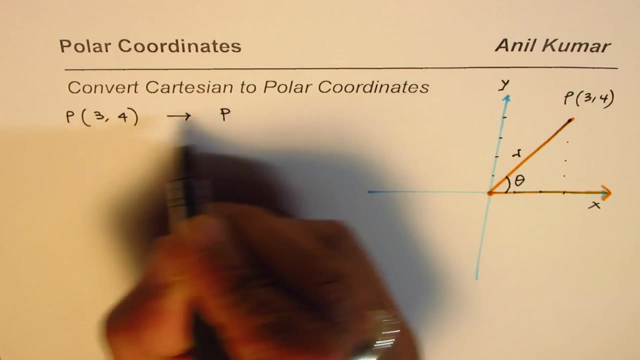 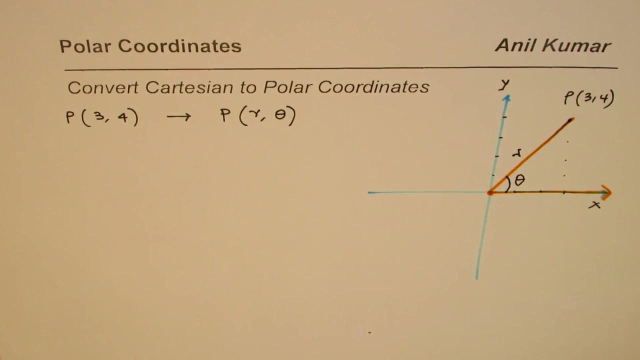 So simple, Where this value is r for us and this angle is theta for us. So we converted this to another point, P, which is actually the same point written as r- theta. Well, now the question is: what is the value of r and what is the value of theta? So that is what we mean when we say 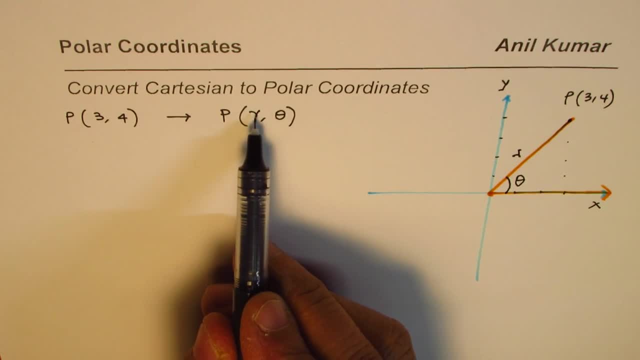 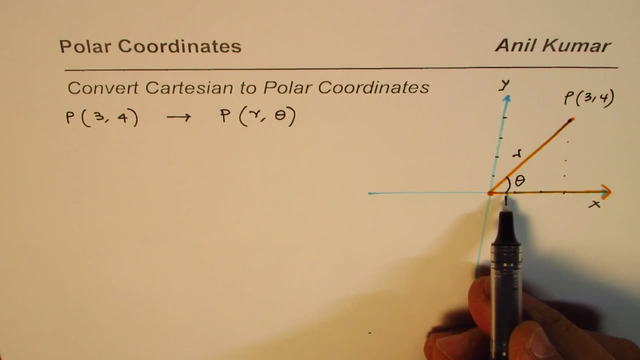 convert cartesian to polar coordinates. That means find the value of r and find the value of theta. theta- distance from the pole, and the counterclockwise angle, theta. this is what we want, right? let us see how to calculate this. now we'll do a bit of construction. take you back to. 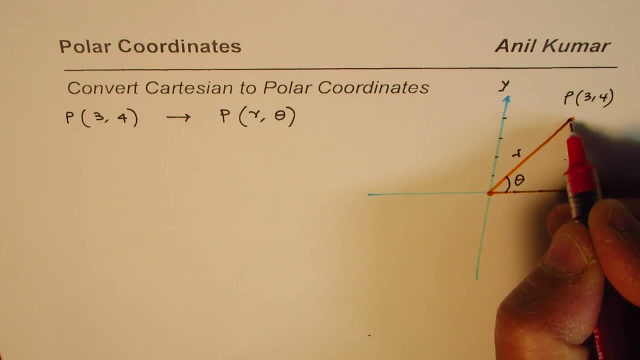 trigonometry, okay, and then we will do the neat form. so this is a kind of to teach you what are the steps involved. so I'm dropping a perpendicular from here to the x-axis that forms the right triangle, correct? and, as you know, this distance here is x value, which is three units, and that is. 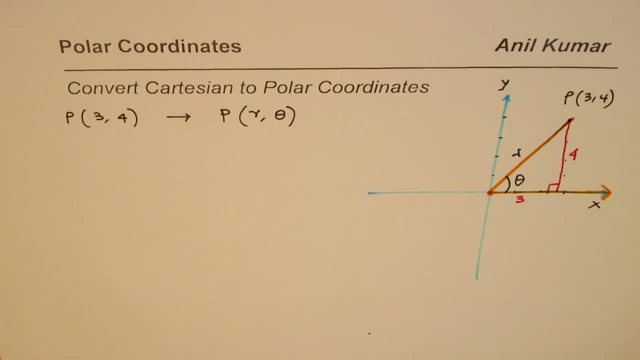 four units. is that okay? now, in general, let's take a general description and then we'll do this particular equation also in general. any point p, which is x and y. so if I replace this point with x and y, in this case that value will be x and this value will be y, correct? So in that case we can. 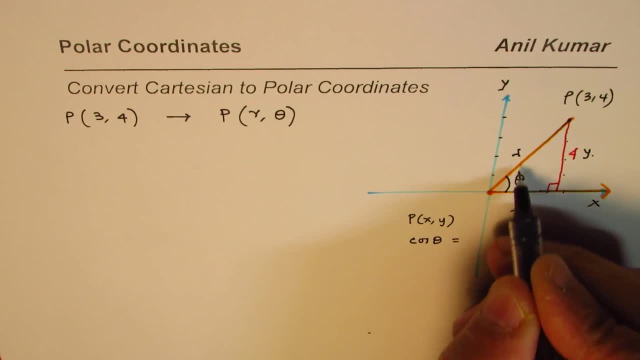 write cos of theta as equals to x over r right, x over r. So that gives me the value of x as equals to r times cos theta right and the value of sine theta is equals to y over r. that means that the value of y could be written as r times sine theta. Using Pythagorean theorem we can write r square. 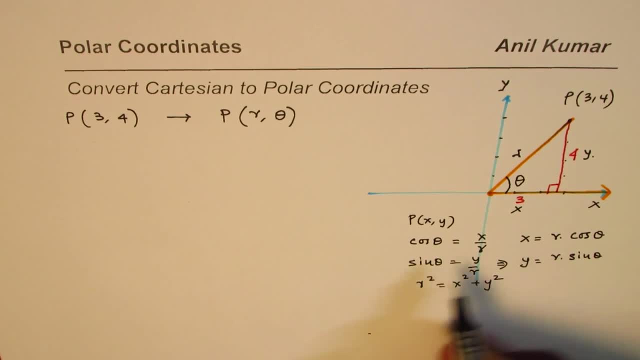 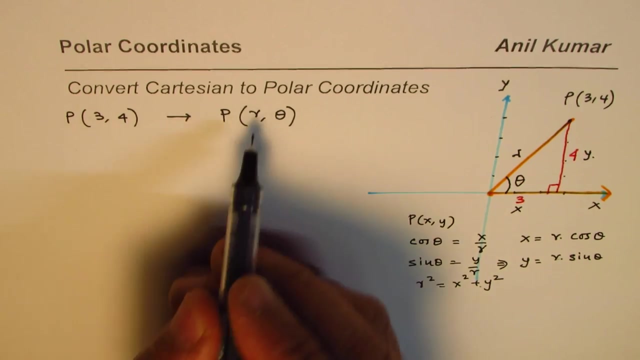 equals to x square plus y square. So what we have done here is we have converted x, y's to r and theta's, and that is what is polar coordinate system, right? So we'll apply this knowledge and then find what r is and what theta is. So what is r equals to? So, as you can see from this, 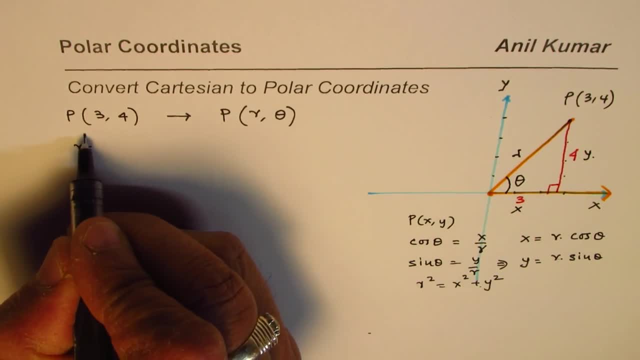 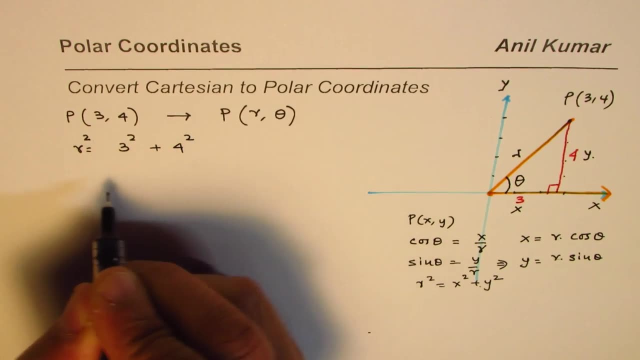 right triangle, r is equals to- rather- let's start with r- square equals to 3 square plus 4 square right, the x square plus y square right, So which is 9 plus 16, which is 25.. So I have taken a very simple 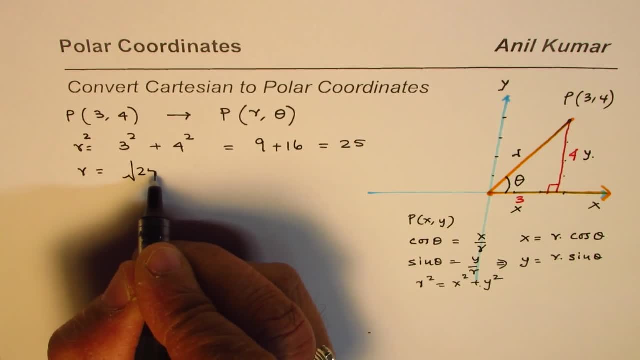 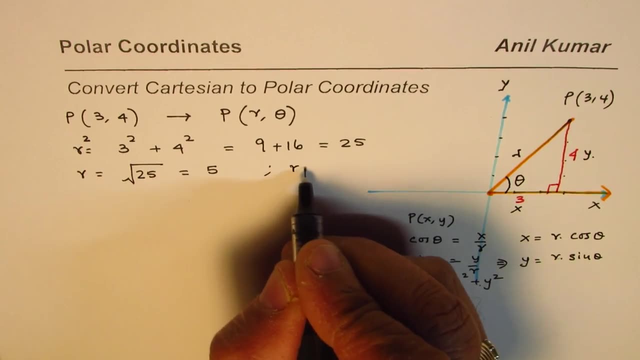 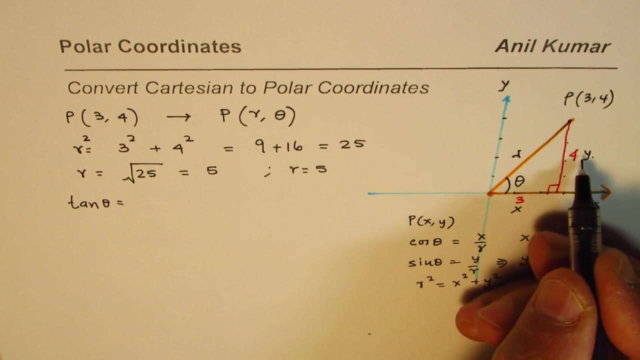 example. So r should be square root of 25, which is equals to 5.. So we know what r is right. So we got r equals to 5.. Now how do you find theta? You use tan theta right. So tan theta equals to y over x or 4 over 3.. So theta equals to tan. 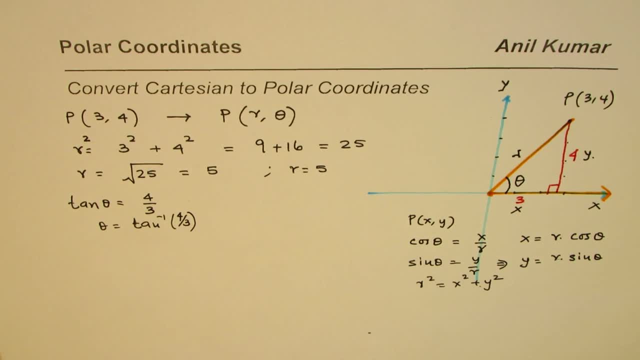 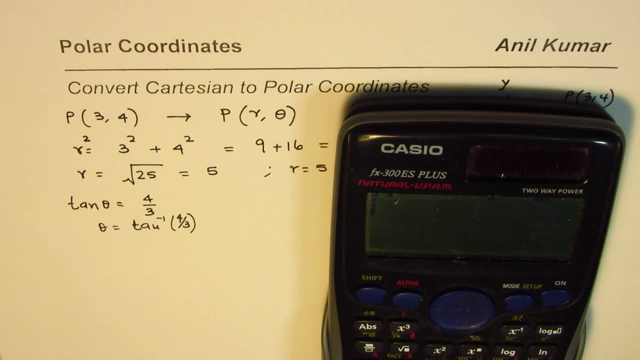 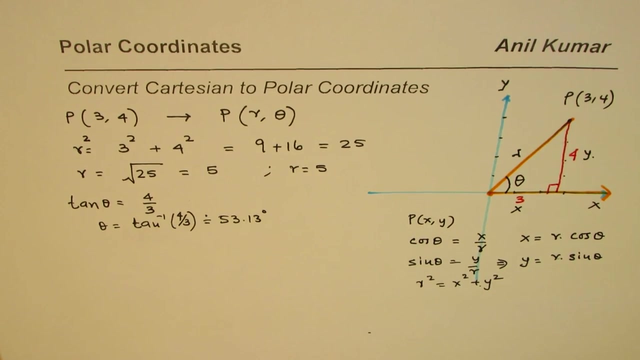 inverse of 4 over 3.. So that is the value of theta. At times you can use calculator to find this approximate value. say inverse tan, inverse 4, divided by 3 equals to: you get 53.130.. Let's say this much degrees approximately, right? So now the answer could be written as point p? r.